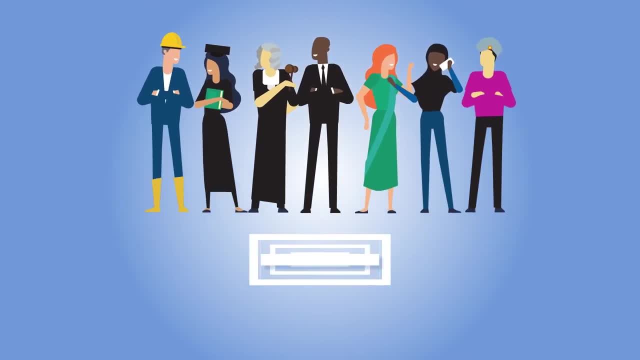 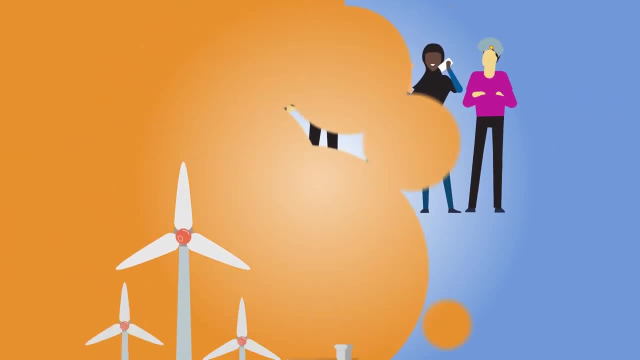 local communities and other data users, all of which, in the years and decades to come, will put the sector under more scrutiny than ever before. Clearly, there is a need not just for progress, but also more transparency on day-to-day operations. the energy transition. 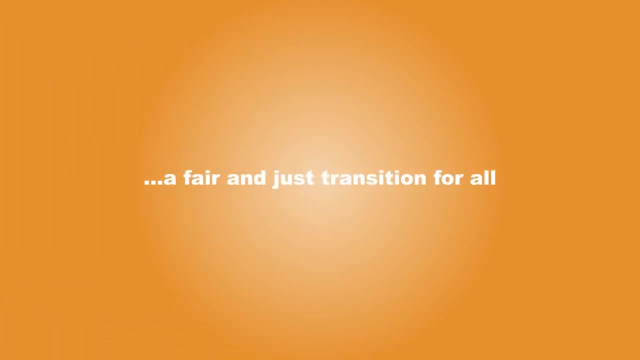 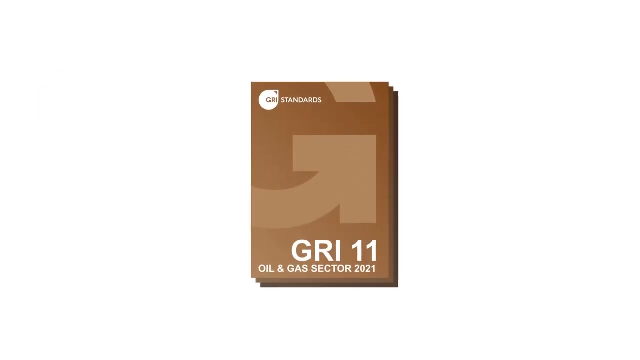 and what will make a fair and just transition for all. GRI has responded to the demand for a new energy-based economy and has been working tirelessly to implement the new standard. Our platform is funded with the launch of a Sector Standard for Oil and Gas: a new global 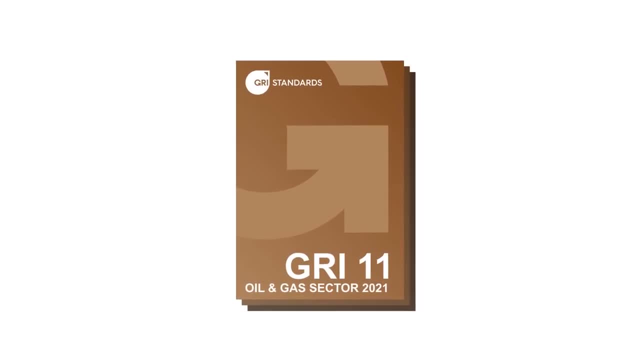 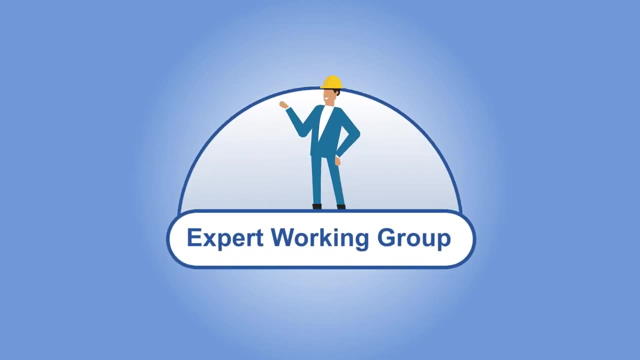 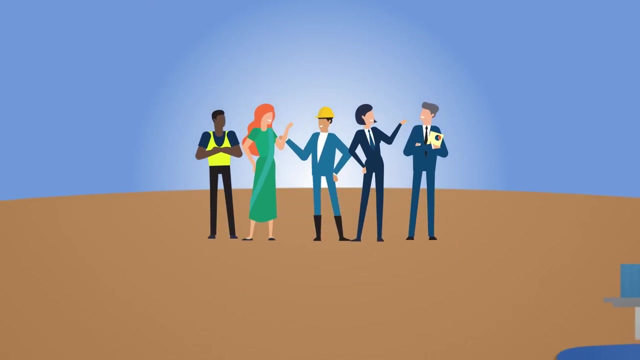 standard that delivers full transparency on the increasingly complex web of oil and gas impacts. We've developed the standard with an expert working group made up of oil and gas companies, investors, civil society, mediating institutions and labor bodies. This means the final GRI standard has unique legitimacy, independent of any one interest group, and enables any company 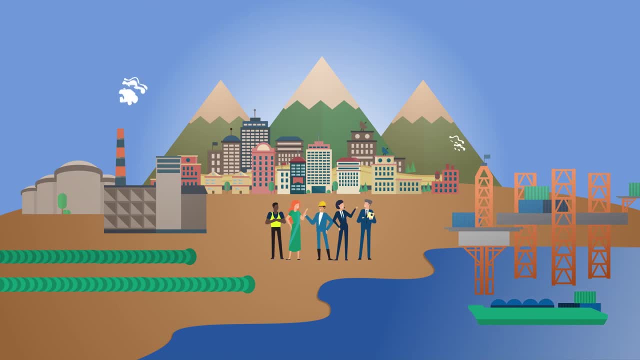 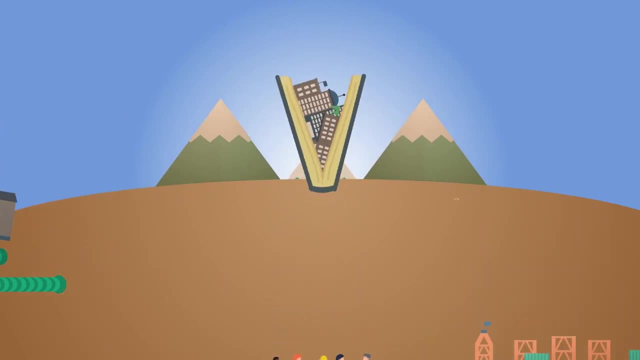 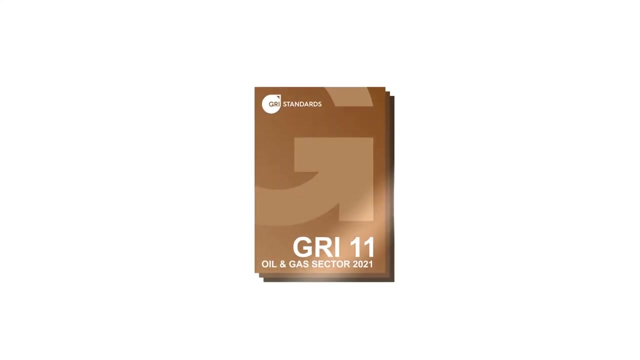 company in the sector to demonstrate accountability by reporting in a consistent and comparable way, while addressing the growing demands of multiple stakeholders. This is a FIRST, a Global Sector-Specific Reporting Standard shaped by sustainable development expectations established for oil and gas, including the EITI standards, the Voluntary 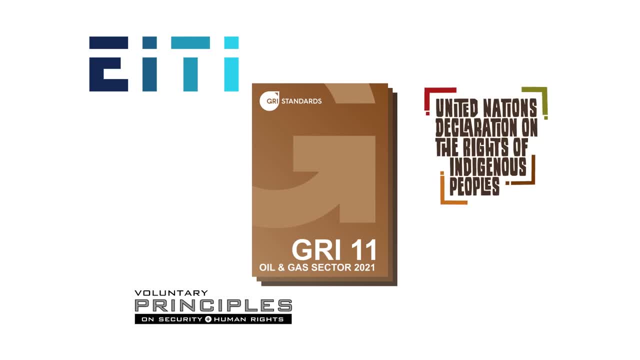 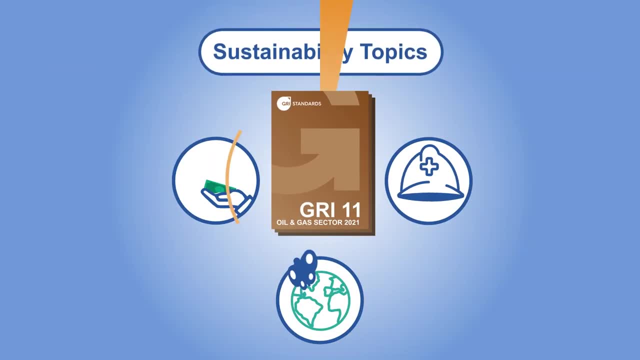 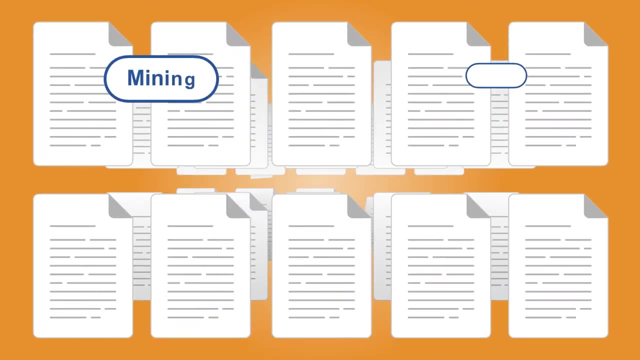 Principles on Security and Human Rights, the UN Declaration of the Rights of Indigenous Peoples and others. It covers the entire scope of sustainability topics. It's also the first of 40 GRI Sector Standards that are to come, which will cover mining, coal, food, textiles, banking and many more. 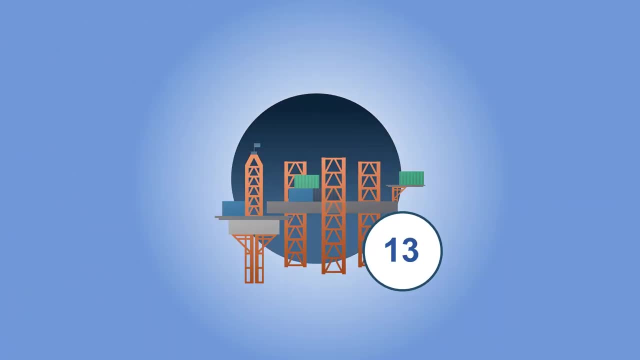 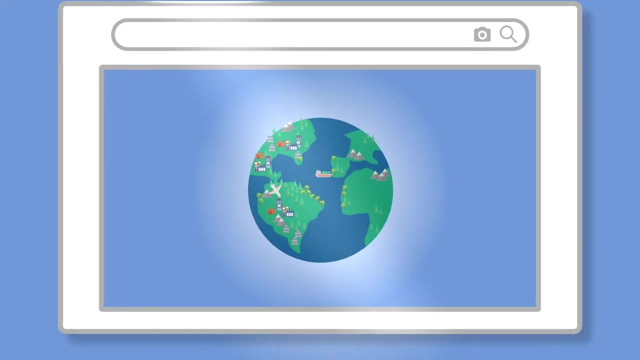 So what do you need to know now? If you are one of the more than 150 oil and gas companies already reporting with GRI, then New Sector Standard is available to use today, Whatever your location, whatever the size of your organization, if you're not already. 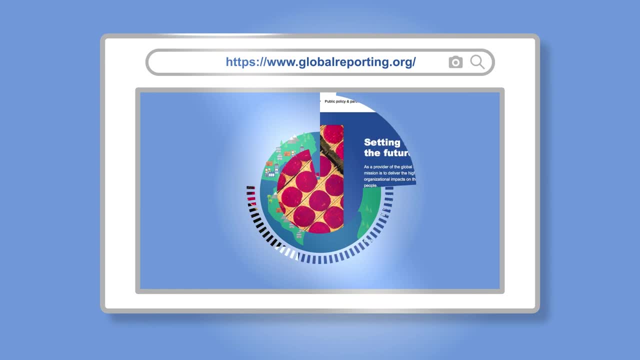 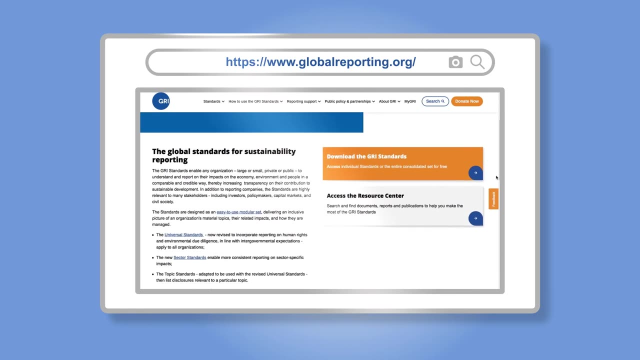 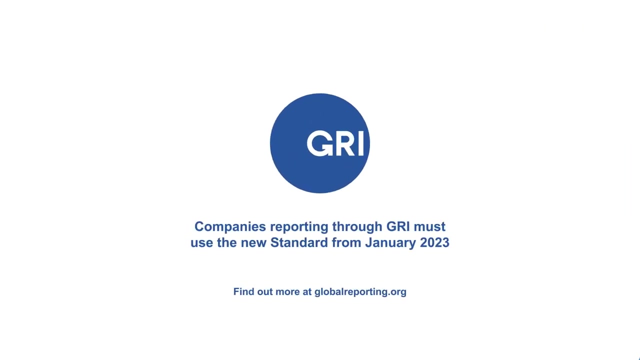 using GRI. you can find out more at globalreportingorg, where you can also discover how the Sector Standard works, alongside our updated Universal Standards, as well as our Topic Standards. Let's get this started and deliver a new era of transparency for oil and gas. New Sector Standard.